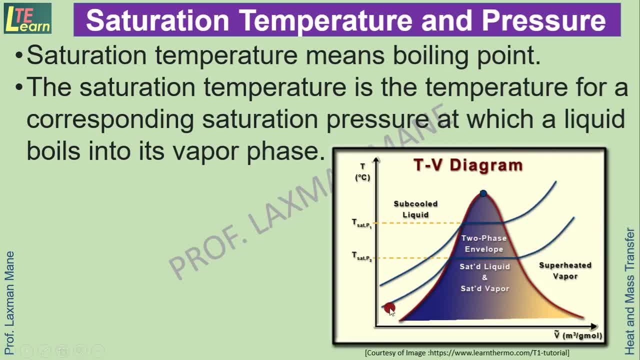 So here this whole region is divided into three parts by this Dome or bell shaped curve. Left side curve is called a saturated liquid line And right side is called a saturated vapor line. These are constant pressure lines, So if the water is heated at some pressure, say atmospheric pressure, 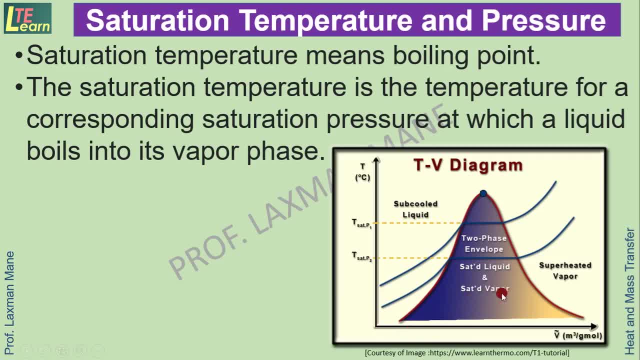 So its temperature will be increased from the ambient temperature To the 100 degree Celsius temperature, That is saturation temperature of the water. So at this point left side water will start to convert into vapor. As the process is continued up to this point, completely that water will be converted into vapor. 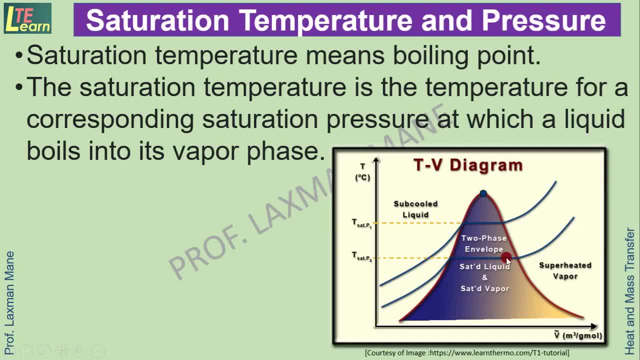 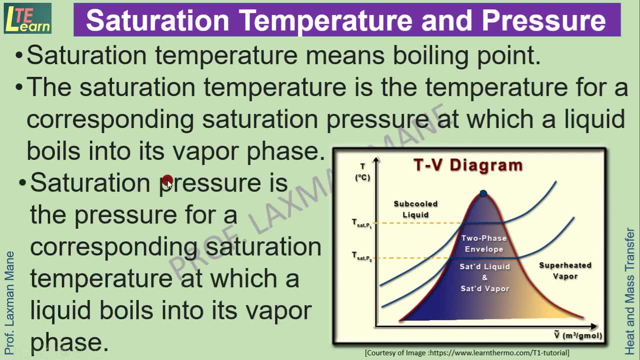 So this process is called as boiling process. Boiling process which is taking place at constant temperature and constant pressure. So saturation pressure is the pressure for a corresponding saturation temperature at which a liquid boils into its vapor phase. What is difference between boiling and evaporation? 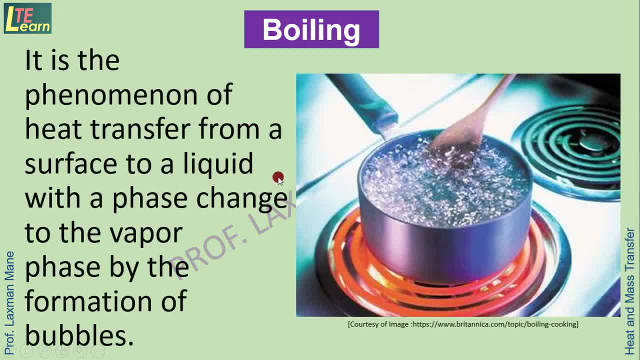 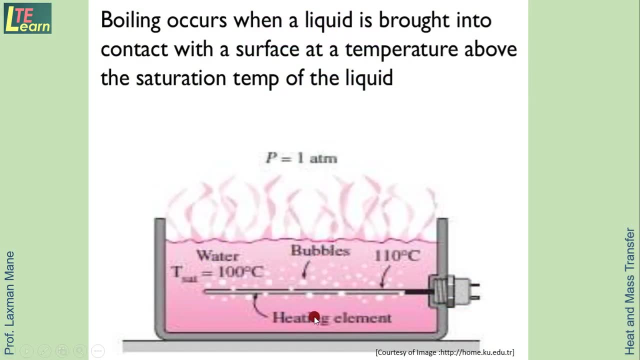 Boiling is the phenomenon of heat transfer from a surface to a liquid with a phase change to the vapor phase by the formation of bubbles. Boiling occurs when a liquid is brought into contact with a surface, For example surface of heater, which is at a temperature above the saturation temperature of the liquid. 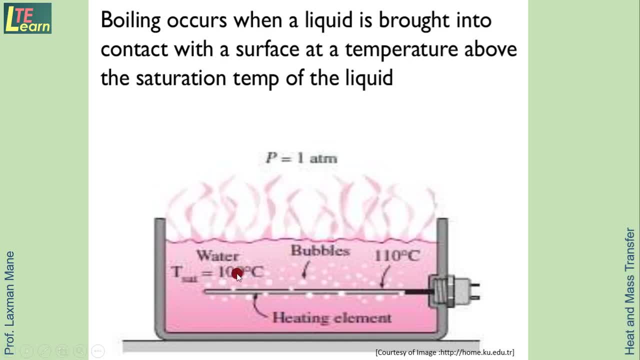 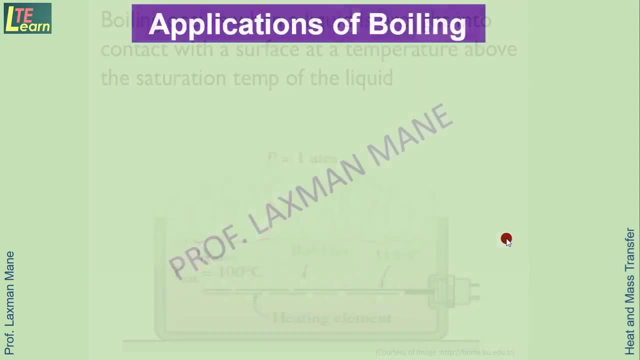 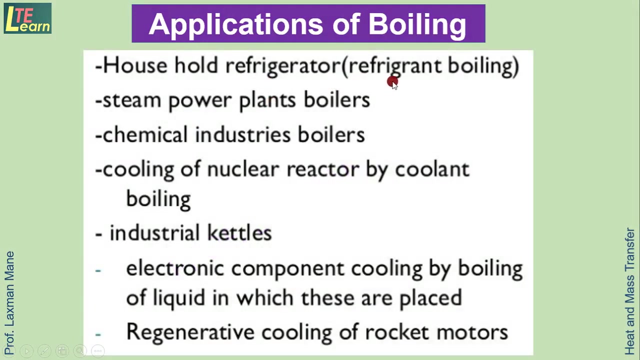 For example, here saturation temperature of water is 100 degree Celsius, Then heater temperature is above 100 degree Celsius, So in that case here boiling occurs. Applications of boiling are in case of household refrigerator, When the refrigerant comes in a few operator coil. 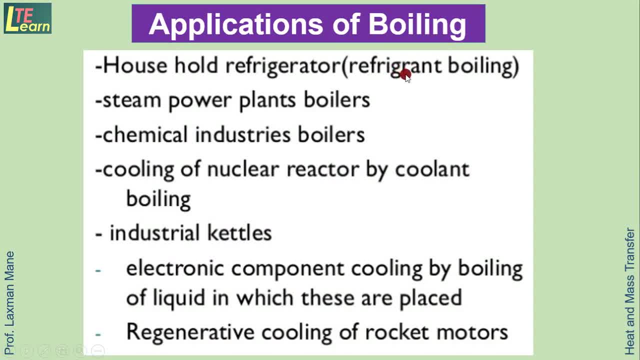 Because of low boiling point, Refrigerant absorb heat from the space to be cooled. Thus liquid refrigerant inside the few operator coil is getting converted into vapor Means. it is getting boiled. In case of steam power plants, Boilers are used to vaporize the water. 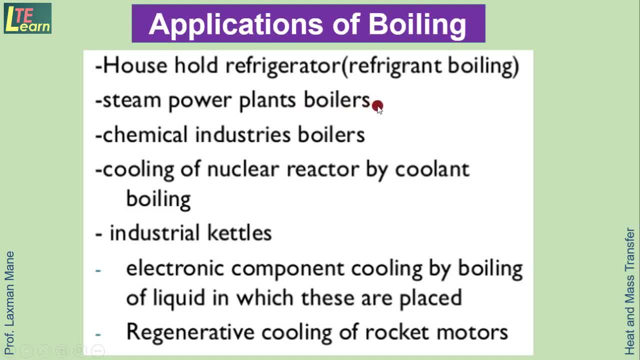 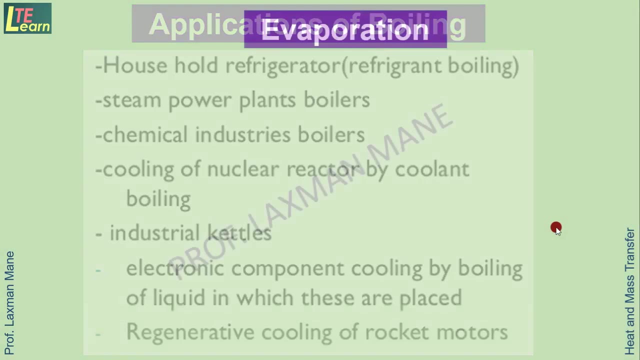 Or to boil the water In order to convert that water into steam. In chemical industries, boilers are used for boiling purpose. In case of electronic component cooling And in regenerative cooling of rocket motors, The process of boiling is utilized. Now we will see about evaporation. 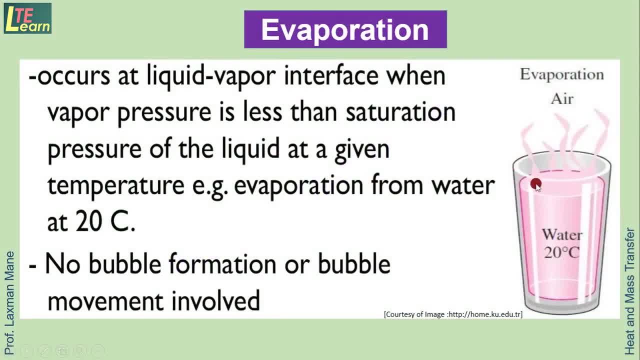 Evaporation occurs at liquid temperature At liquid vapor interface Means at this top surface of water. for example, It happens when vapor pressure is less than saturation pressure. Vapor pressure means pressure applied by the vapor on the liquid surface, So this is at given temperature. 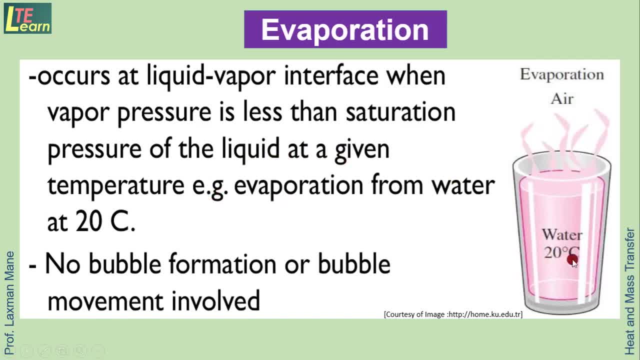 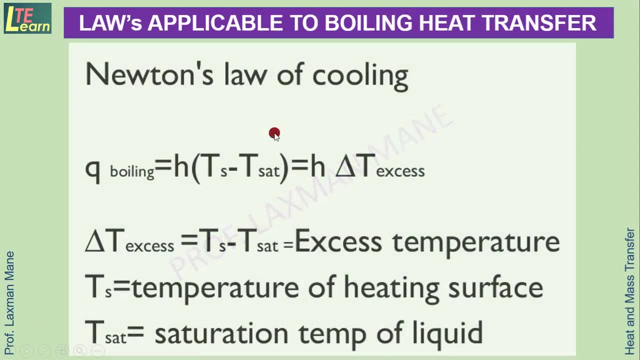 So this is a temperature, for example, 20 degree Celsius. So in this case no bubble formation or bubble movement involved inside the water. Law applicable to boiling heat transfer Is Newton's law of cooling. That already we know. That is equal to H into T S minus T Sac. 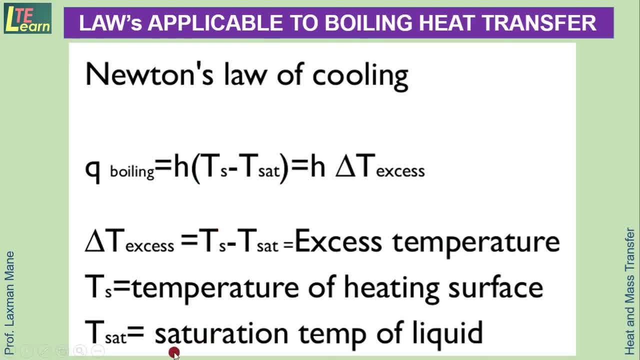 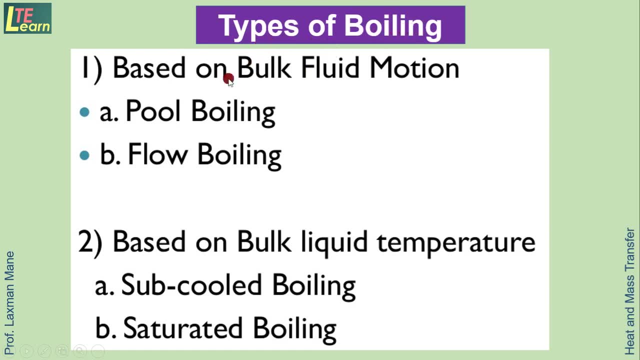 Where T S is the temperature of heating surface And T Sac is the saturation temperature of liquid. This difference is called delta T X- S. So here classification of boiling is based on bulk fluid motion. There are two types: Cool boiling and flow boiling. 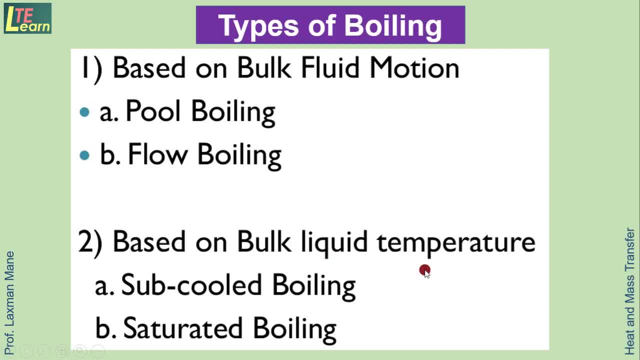 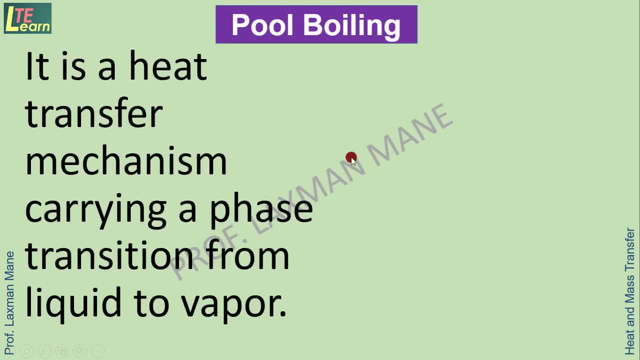 And based on bulk liquid temperature. It is divided into two types: Sub-cooled boiling and saturated boiling. Now we will see, one by one, Each kind of boiling Pool boiling: It is a heat transfer mechanism Carrying a phase transition from liquid to vapor. 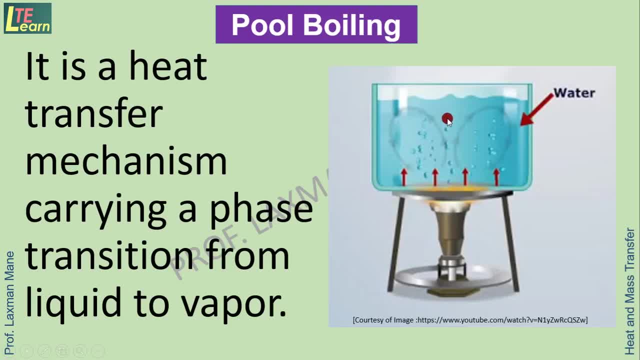 So here we see. This is a water which is kept in a pot And this is application of heat at the bottom. So, however heat is added, Temperature of this water is going to rise. So this whole process of pool boiling is shown. 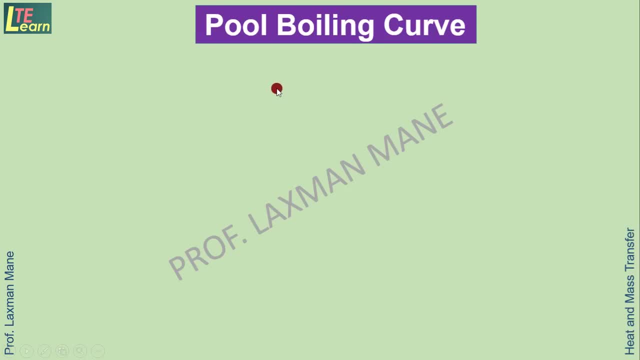 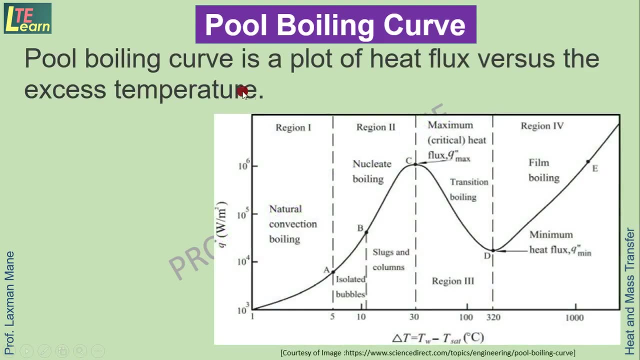 Or expressed by using curve That is called as pool boiling curve. It is also called as pool regime. So this pool boiling curve, This curve which is a plot of heat flux Versus excess temperature, So on Y axis, this is a heat flux. 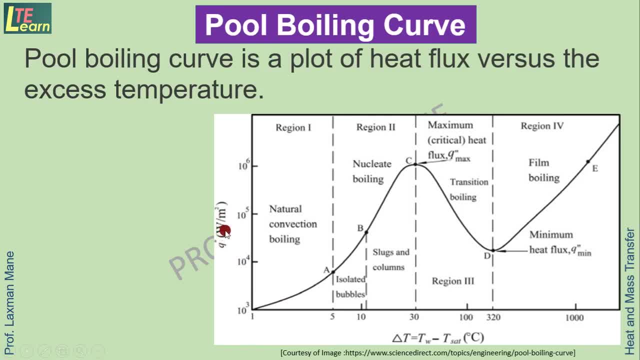 Means Watt per meter square. Watt is a energy Amount of heat transfer divided by area. On X axis this is a temperature difference Between surface temperature and fluid temperature. That is delta T. So this Boiling curve, Pool boiling curve. 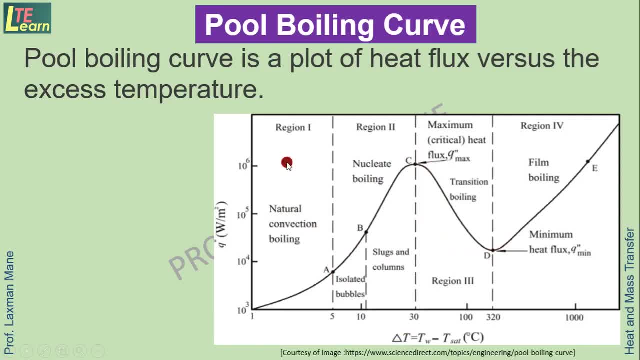 Has four regions. So region first Is called as natural convection boiling. Region second is called as nucleate boiling. In third region Transition boiling is taking place And this is last region. In that film boiling is taking place. Now we will see about each kind of boiling. 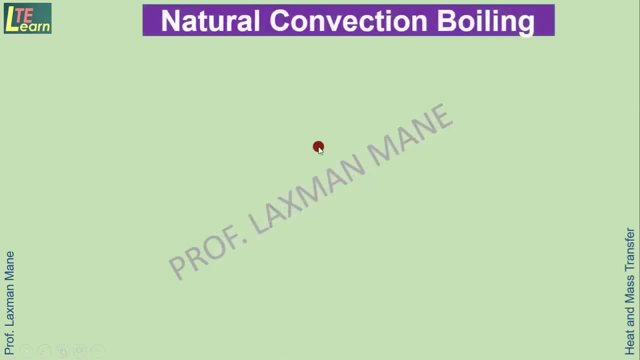 In detail. So natural convection boiling. In thermodynamics The requirement for boiling of pure substances To occur is that Saturation temperature Of the liquid Is equal to surface temperature. But in real experiments Boiling does not occur. 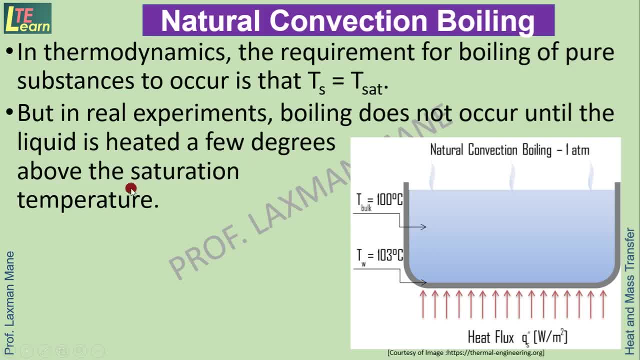 Until the liquid is heated A few degrees above the saturation temperature. So from this diagram you can see The surface temperature is Greater than the Saturation temperature of liquid For one atmosphere. Saturation temperature of Water is 100 degree Celsius. 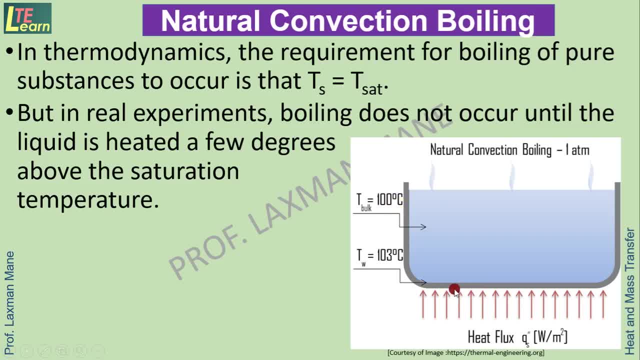 So this Surface temperature Is more than 100.. Say here is considered as 103 degree Celsius. So this difference, That we say delta T excess In case of natural convection boiling, Is less than 5 degree Celsius. 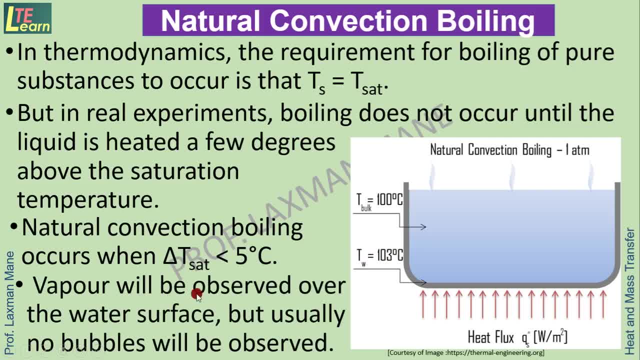 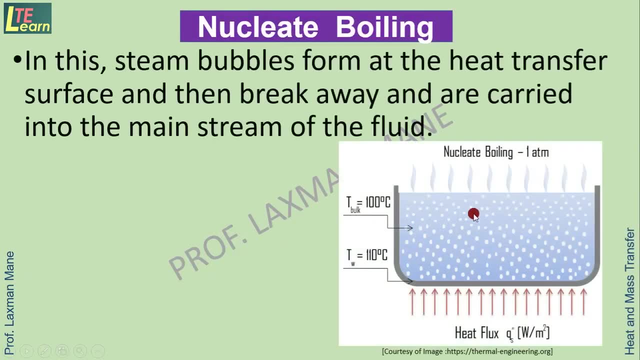 So in this case Vapor will be observed Over the water surface, But usually no bubbles Will be observed inside this Water Nucleate. boiling In this Steam, bubbles form At the heat transfer surface And then break away. 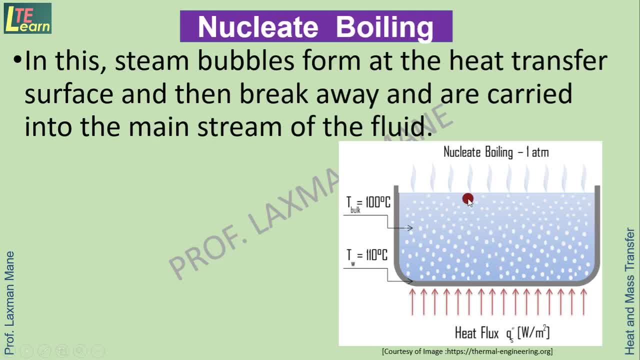 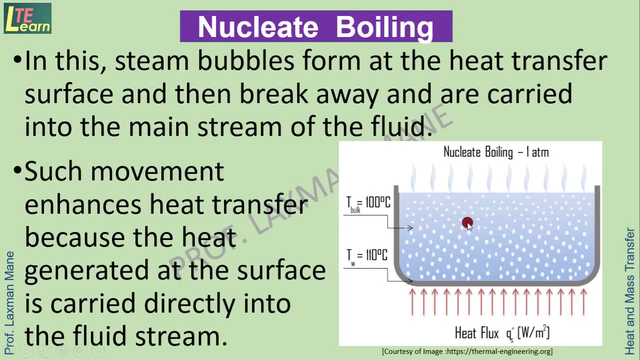 And are carried Into the main Stream of the fluid. So here, This surface temperature Is more than Saturation temperature. So here, This moment Of this bubbles enhances Heat transfer, because The heat generated at the surface Is carried directly. 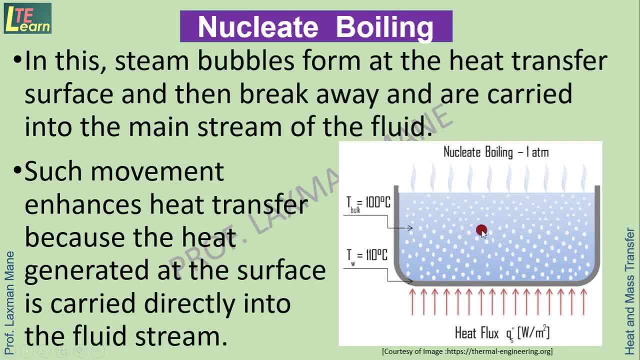 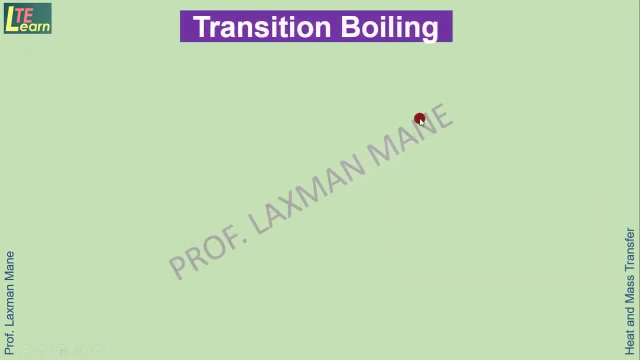 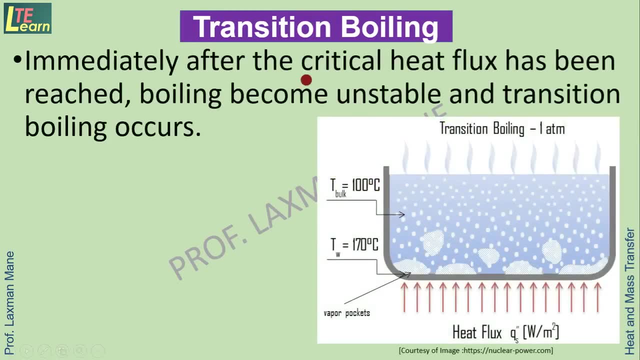 Into the fluid stream By the bubbles which are forming. That is What Nucleate boiling, Transition boiling. That is happening in third region Of the pool boiling curve, So immediately After the critical heat flux Has been reached. 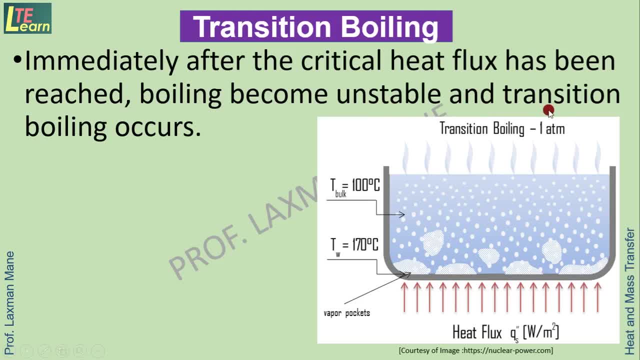 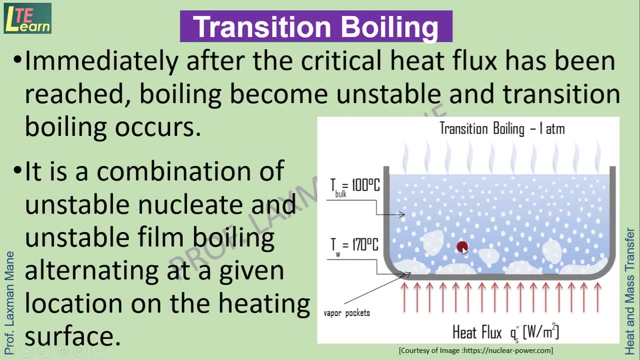 Boiling becomes unstable In this region And transition boiling occurs here. So in this case Delta T excess is more You can see here. So Transition boiling is a combination of Unstable nucleate And unstable film boiling. So transition boiling is a combination. 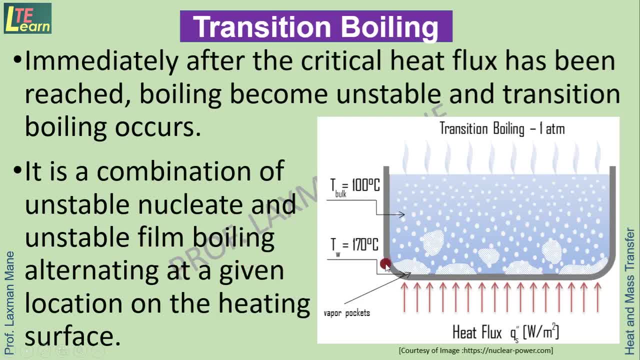 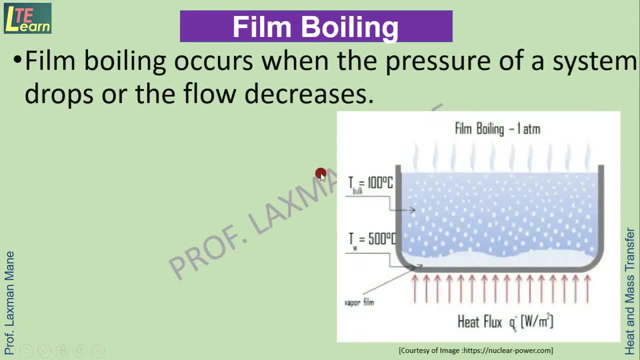 Of sixth, Third and fourth region. Last region is Of film boiling. So film boiling occurs When the pressure of a system drops Or flow decreases. In this case the bubbles cannot escape As quickly From the heat transfer surface. So this is a heat transfer surface. 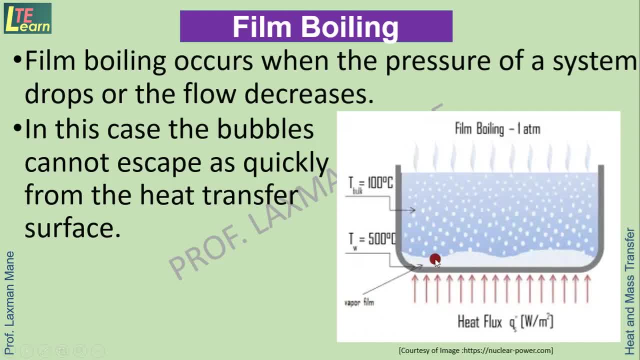 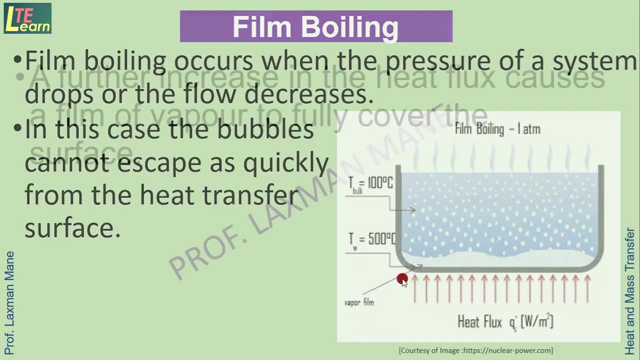 So here you see, Vapour film is Developed, And above vapour film, These are the bubbles Which are escaping From this vapour film, But these are not escaping From the heating surface. A further increase In heat flux. 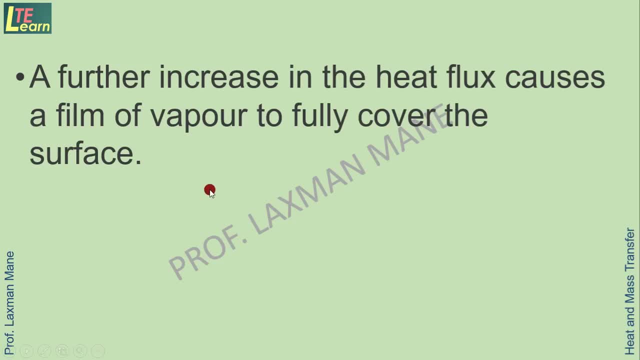 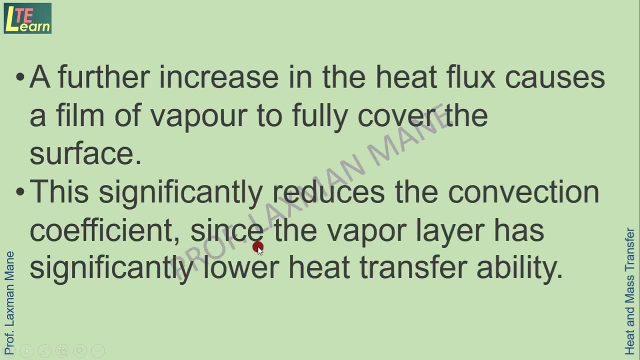 Causes a film of vapour To fully cover the surface, Which is the reason Of formation of film. This significantly reduces The convection coefficient. Means H, Since the vapour layer Has significantly lower Heat transfer ability. Next, type of boiling: 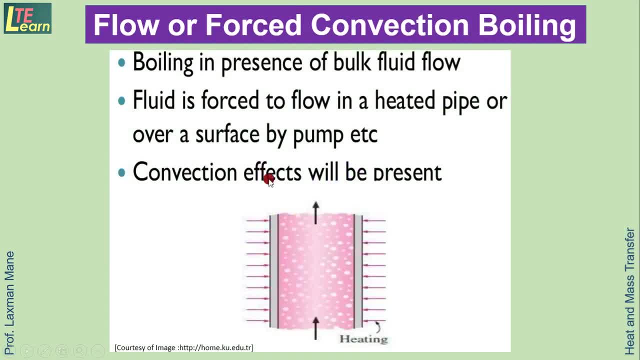 Is flow Or forced convection boiling. In this case, boiling Happens in presence Of bulk fluid flow Which is taking place Through this pipe Or over a surface. The fluid is forced To flow Through this pipe or surface. 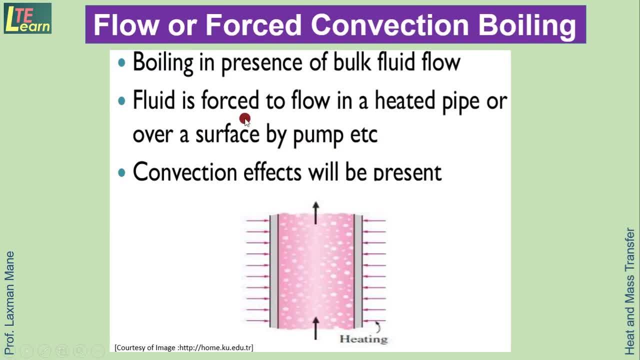 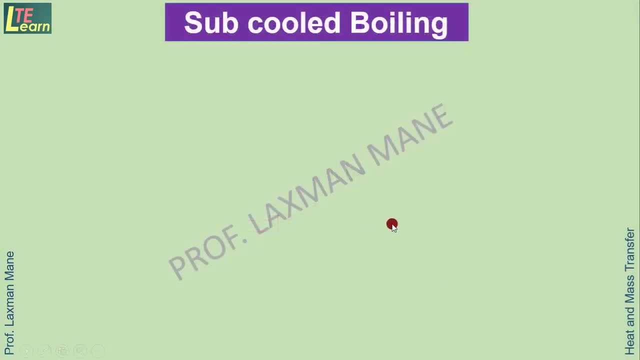 By pump. So this is an external agent Or external mechanical component, As a pump is here To force the fluid, So in this case convection Effects will be present. Sub cooled boiling. In this Sub cooled means The left side region. 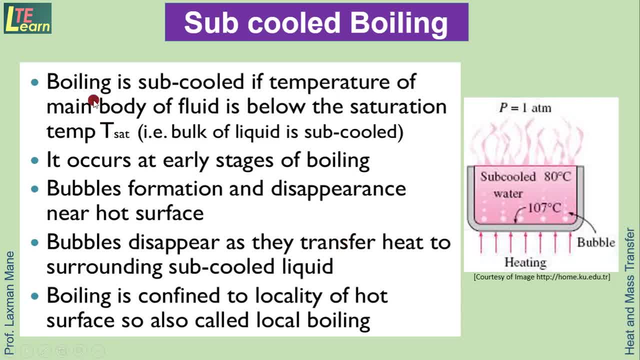 Is sub cooled region. So in this case The boiling is sub cooled If the temperature of main body Of fluid Means temperature of liquid, That is saturation temperature, That is Less than the Bulk of liquid. So here you see. 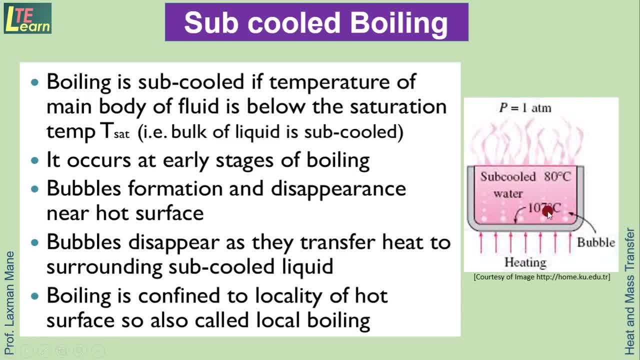 Sub cooled water. That is at 80 degree Celsius And this is 107 degree Celsius. That is surface temperature, So saturation temperature is Lower than the surface temperature. It occurs at Early stages of boiling, In this case Bubble formation and disappearance. 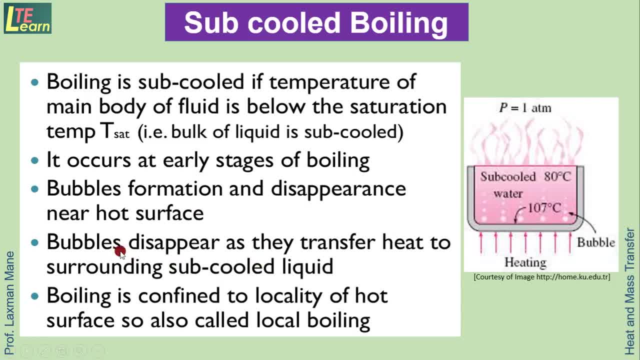 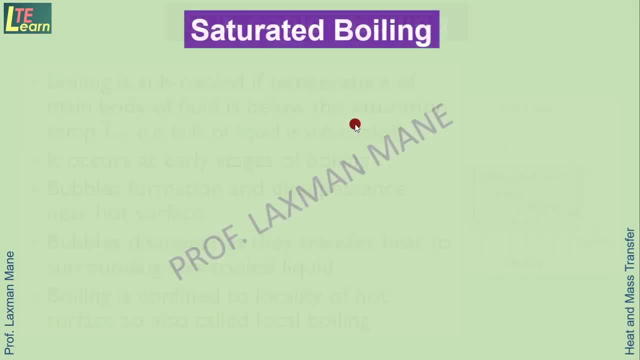 Near the hot surface occurs, Bubbles Disappear as they transfer heat To the surrounding Sub cooled liquid. This is Also called as local boiling, Because it is taking place On the surface. Saturated boiling, Which take place at: 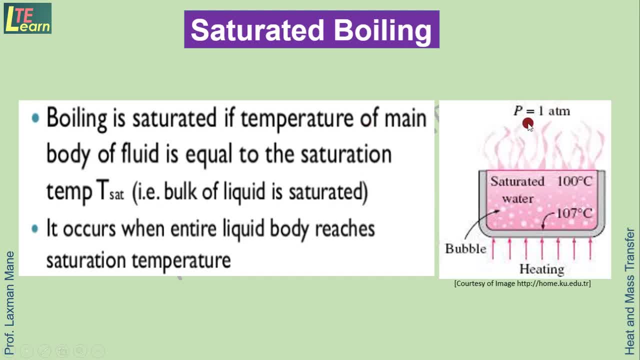 Saturated temperature. For example, In case of water Atmospheric pressure Saturation temperature is 100 degree Celsius, So boiling is saturated In this case If the temperature of main body of fluid Is equal to saturation temperature. Now the second part. 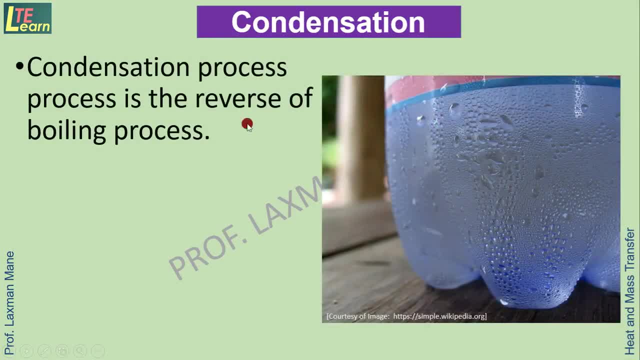 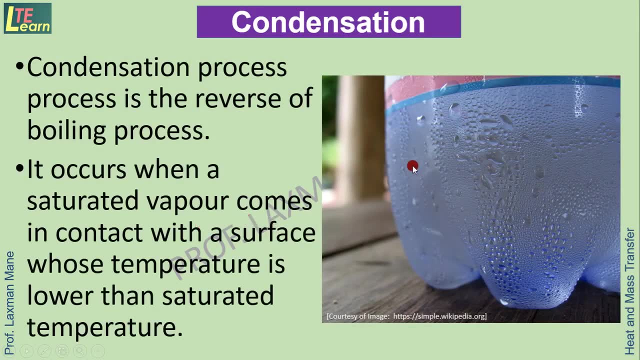 Condensation. Condensation process Is the reverse of boiling process. It occurs When a saturated vapor Comes in contact With a surface Whose temperature is lower than Saturated temperature. So, for example, here This is a bottle shown. 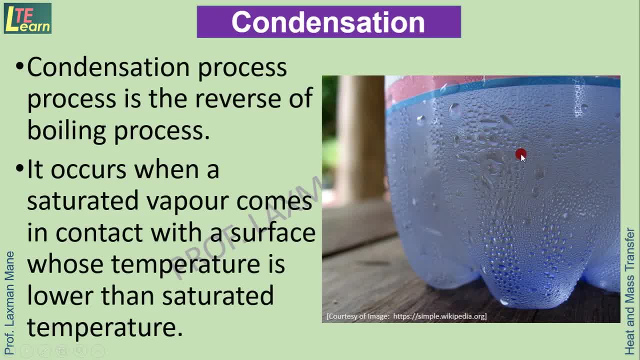 Inside this bottle the fluid or liquid is present. Its temperature is Lower than The saturated temperature. That's why here The outside Vapor present in the air, When comes in a contact with this Bottle, Condensation is taking place. 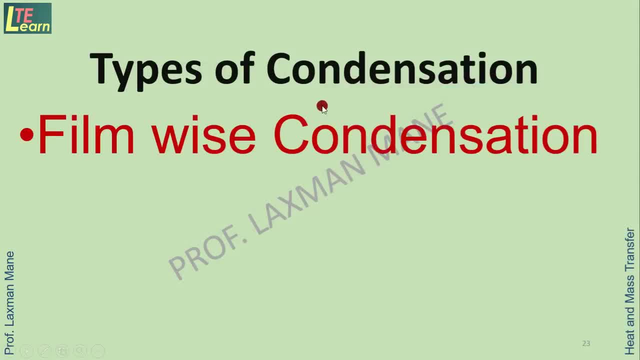 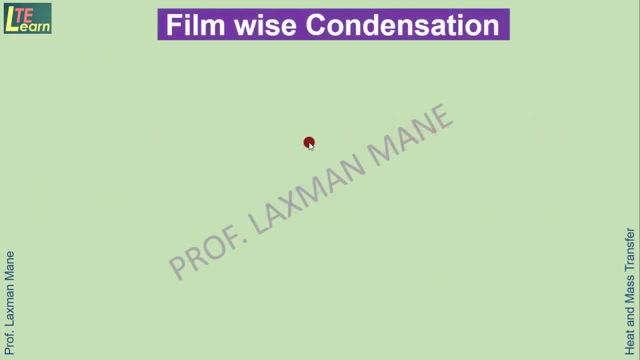 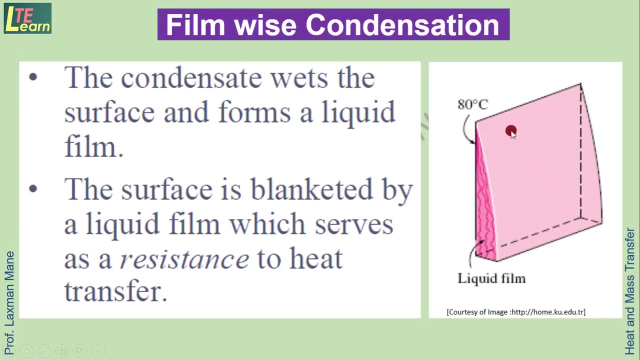 Now there are two types Of condensation. First is a film wise condensation And second is Drop wise condensation. In case of film Wise condensation, The condensate wets The surface Is a liquid film. 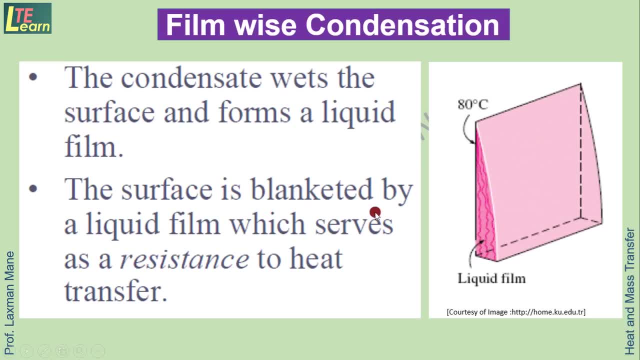 So this is a liquid film Which is forming. The surface is Blanketed by a liquid film Which serves as a Resistance to heat transfer. So by this, Heat transfer is reduced Because of this film. Liquid film, Second, is a drop wise condensation. 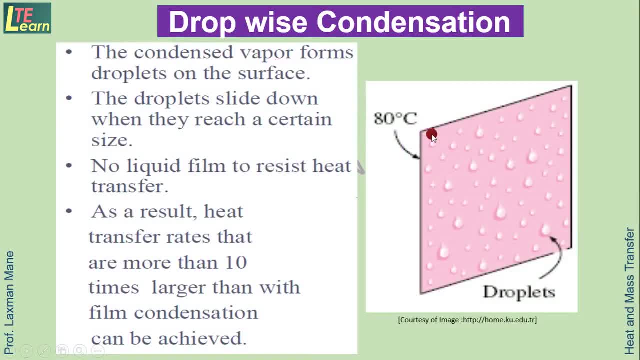 Here, The condensed vapor Drops droplets On the surface. The droplets slide down When they reach A certain size. No liquid film Here to resist heat transfer. Thus, As a result of this, Heat transfer rate Is, in this case,